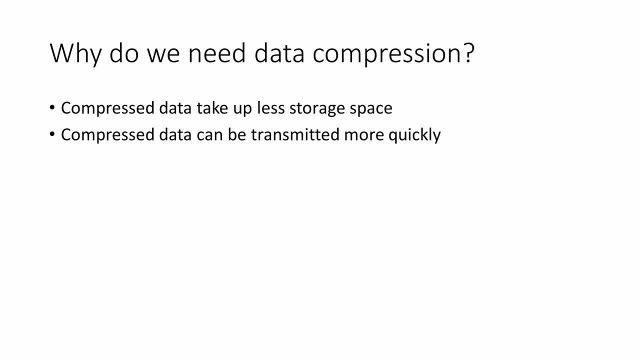 can also speed up data transmission. A data compression program converts data from a ready-to-use format into a format optimized for compactness. A decompression program returns the compressed data back into its original form. There are two main categories of data compression: lossless and lossy. Suppose, for example. 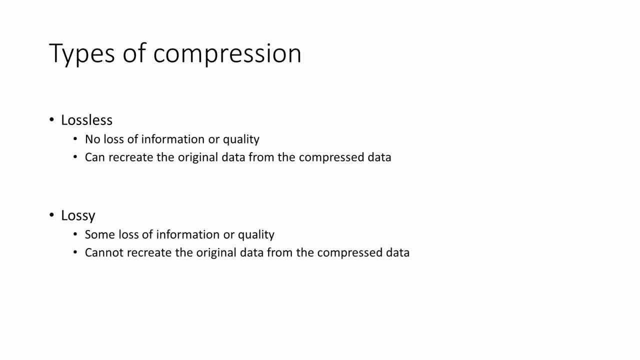 you are compressing an image or a video file. Lossless compression means that the compressed file contains all of the information needed to recreate the original file without any loss of quality. When the file is decompressed, the image or video will look as good as the. 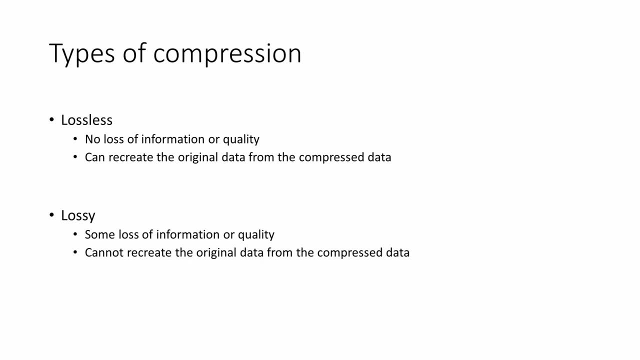 original Lossy. compression, on the other hand, means that when the compressed file is decompressed, it will not contain the same amount of data as the original. Some of it is lost and the image or video may not look quite as good as the original. 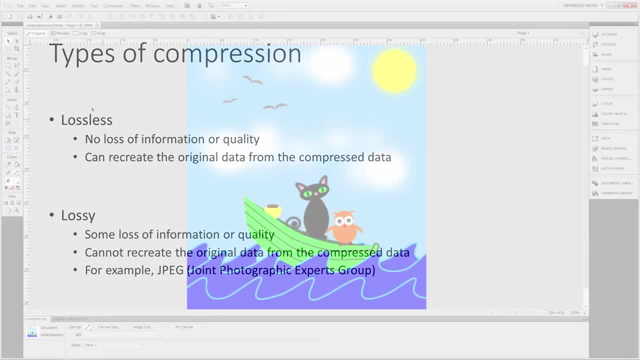 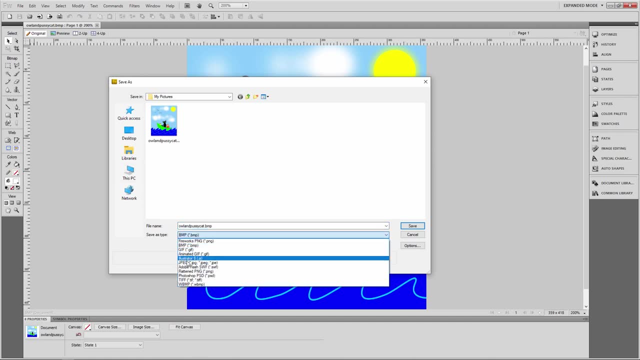 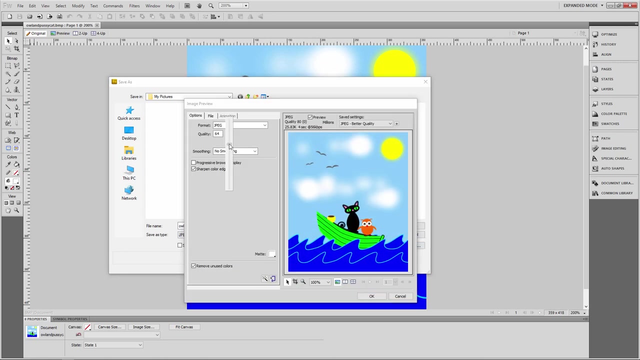 JPEG is a widely used lossy compression format for images. You can use a graphics application like Fireworks or Photoshop to save an image as a JPEG and you can control the amount of compression. Usually, it is possible to strike a good balance between a reduction in file size and 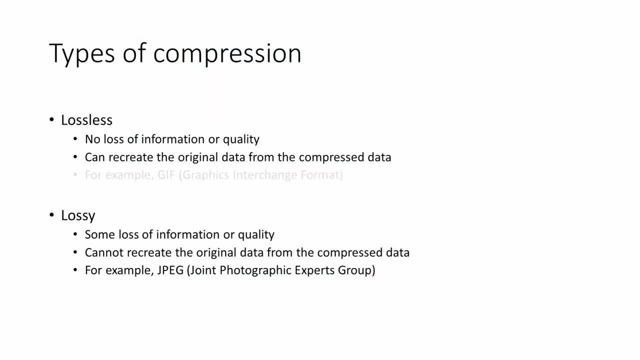 the permanent loss of quality it will cause. GIF is a widely used lossless compression format for images. JPEG is the best choice for digitized photographs, while GIF is more often used with simple drawn images such as logos that have large areas of a single color. When it comes to textual data such as a document or a computer program, lossless compression is the best choice. When it comes to textual data, such as a document or a computer program, lossless compression is the best choice. JPEG is the best choice for digitized photographs, while GIF is the best choice for. 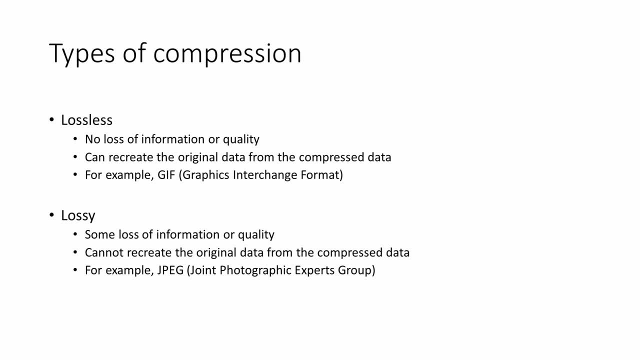 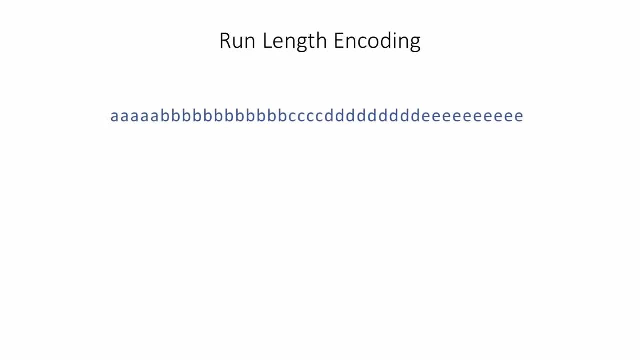 Lossless compression is essential, otherwise the decompressed document will be unreadable. Now let's talk about how compression works. There are lots of different techniques in use. In fact, some of the most well-known compressed formats, such as JPEG, employ a combination. 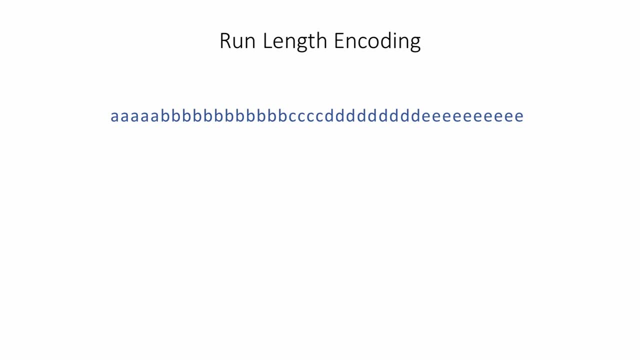 of techniques. One of these techniques is known as run-length encoding. Consider this block of data. Perhaps it was generated by some sort of poll or survey, or perhaps it's the output of some kind of data logging application. Whatever the case, this is a good candidate for compression by run-length encoding. 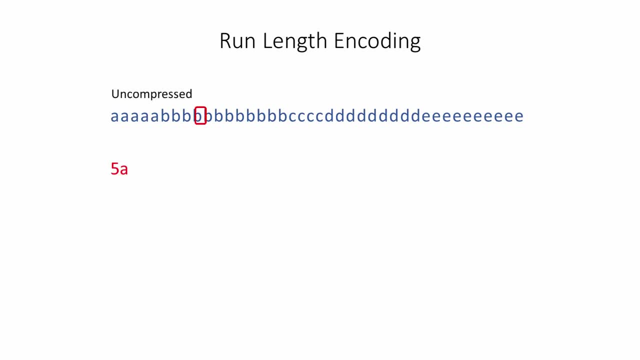 The essence of run-length encoding is to scan the data you want to compress and, for each item, record the run-length, that is, the number of times it occurs, followed by the item itself. In this example, there are five A's. 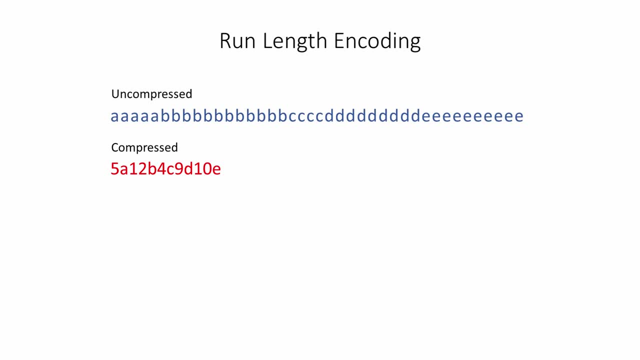 Twelve B's, four C's and so on. Notice that the compressed dataset is about a quarter of the size of the original Run-length. encoding is a lossless form of compression because the compressed dataset contains everything necessary to recreate the original data. 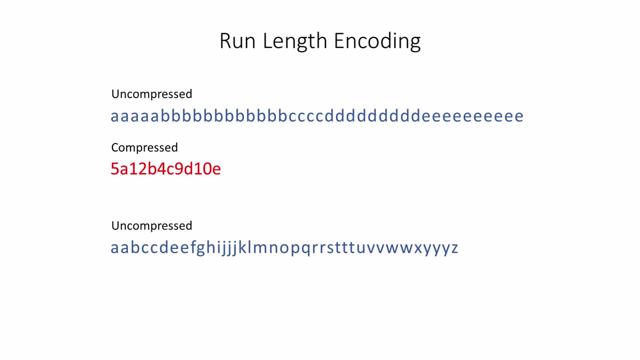 Now consider this uncompressed dataset. There's a lot more variation in the data this time. Indeed, the compressed form of the data is larger than the uncompressed form. Compression has actually made the situation worse. This is called negative compression. Of course, both of these examples are something of a simplification. 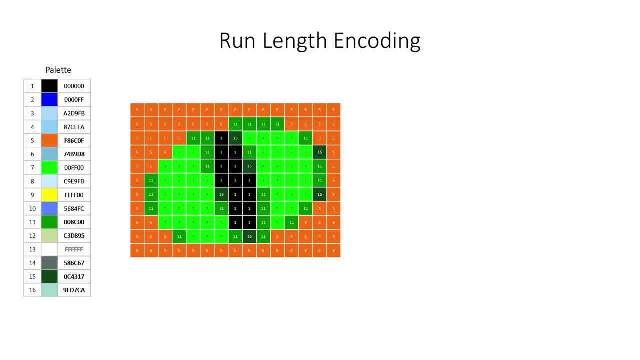 Consider this simple indexed bitmap image, which has a palette of only 16 colours. Because there are only 16 possible colours, the colour of each pixel can be encoded with only 4 bits. The denary values are shown here for convenience. The image has a width of 15 pixels and a height of 11 pixels. 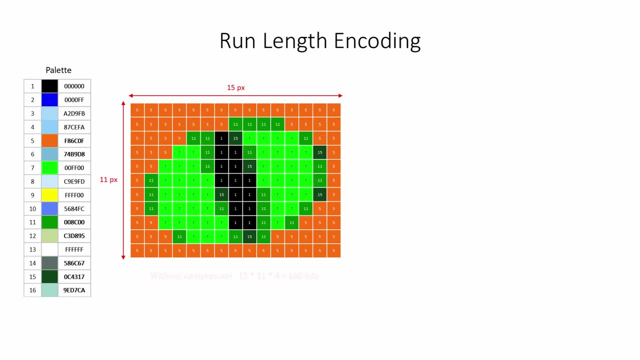 That's 165 pixels altogether. If the colour of each pixel is encoded separately with 4 bits per pixel, the image takes up a total of 660 bits. When run-length encoding is applied, the image is scanned from left to right row by row. 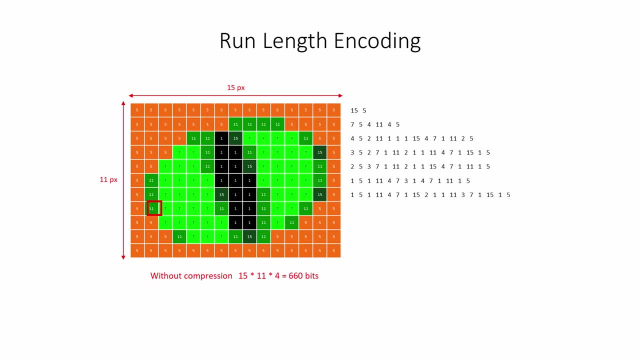 The image is then scanned from left to right, row by row. The image is then scanned from left to right, row by row. Each row is treated separately Whenever there's a change in a pixel value, a run count and the corresponding value is. 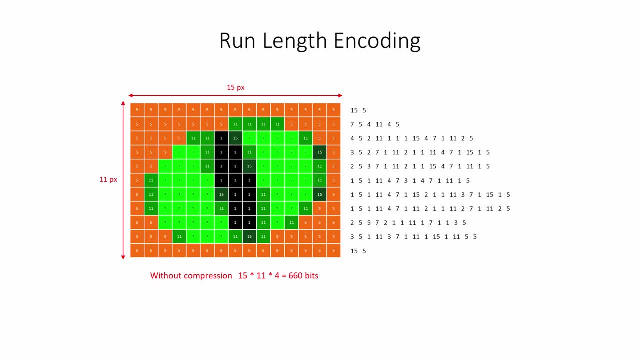 generated. Notice how the first row consists of 15 pixels, each with a value of 5.. The second row starts with 7- 5s, followed by 4, 11s, followed by 4 more 5s, and so on. 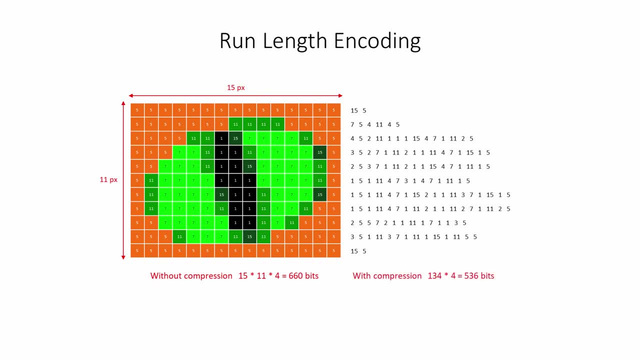 This time, there are 134 data items that need to be stored, instead of 165.. The first row consists of 15 pixels, each with a value of 5.. The second row starts with 7- 5s, followed by 4- 11s, followed by 4 more 5s, and so on. 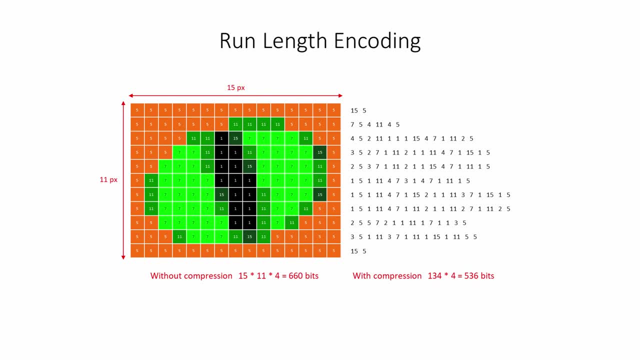 Each of these values can also be encoded with 4 bits, so this time we only need to store 536 bits of data. This is not a huge difference, but consider this simpler version of the same image. using the same palette, There are much longer runs of the same colour this time. 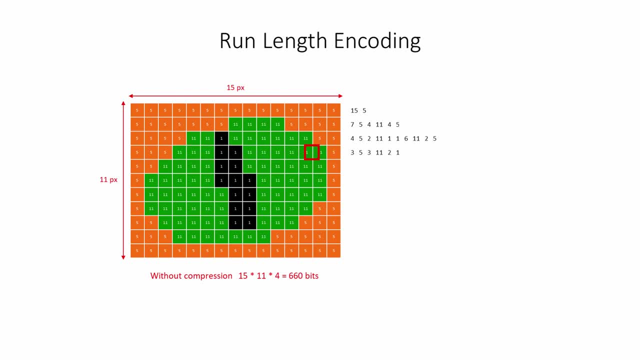 When run-length encoding is applied in the same way, there are only 86 items that need to be saved. As you can see, there are no more runs of the same colour. Assuming each pixel is encoded with 4 bits as before, this makes the compressed image. 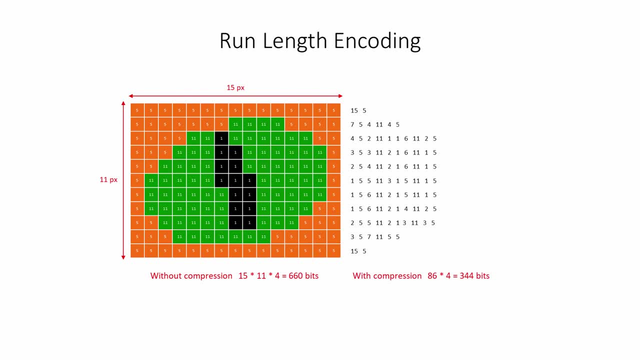 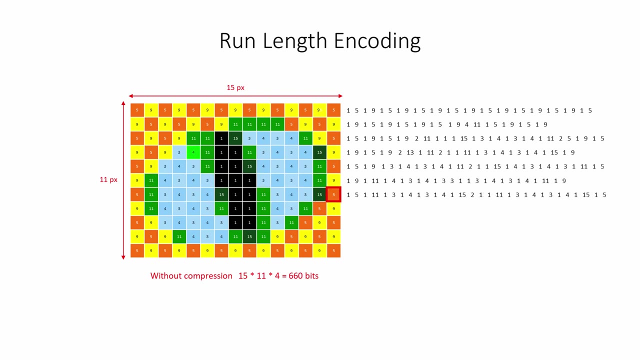 about half the size of the original. However, in a very colourful image with only short runs of the same colour, run-length encoding can produce undesirable results. In this example, run-length encoding generates 311 items that need to be saved. That's nearly twice as many as the original 165.. 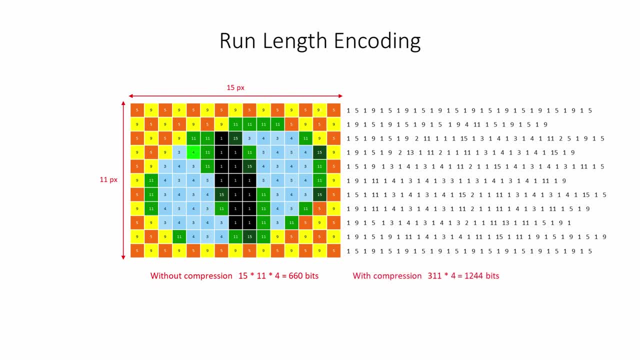 This means that each pixel is encoded with 4 bits. The compressed image file is therefore nearly twice the size of the original. Clearly, run-length encoding is not suitable for all types of image data. We've seen this before. It's known as negative compression. 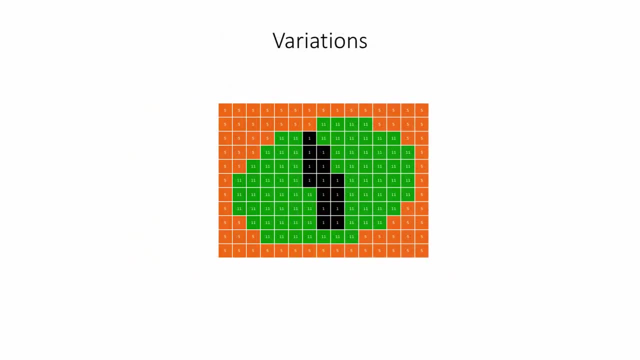 Some implementations of run-length encoding continue counting values in a run over more than one line. For example, this image can be encoded as 22 files. This means that run-length encoding is not suitable for all types of image data. We've seen this before. 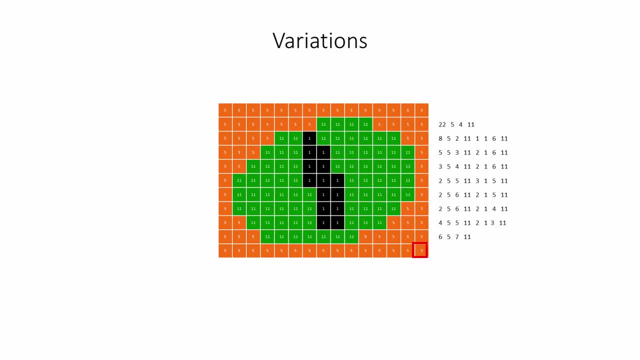 The compressed image file is therefore nearly two times the size of the original 18ff file. The compressed images claim to be 48 files, and these must be finished in a special sentido format. We've seen this before. The compressed image files can be used as: 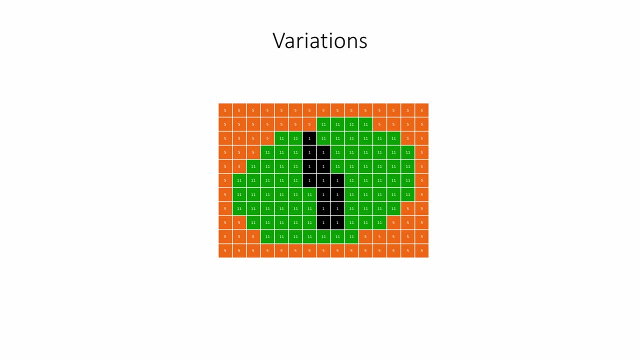 a replacement for a mijn, But we don't think this is right appearance In this case. we want to adjust color column-wise and save the output of whichever approach produces the best result. These days, run-length encoding is rarely used on its own for image compression. 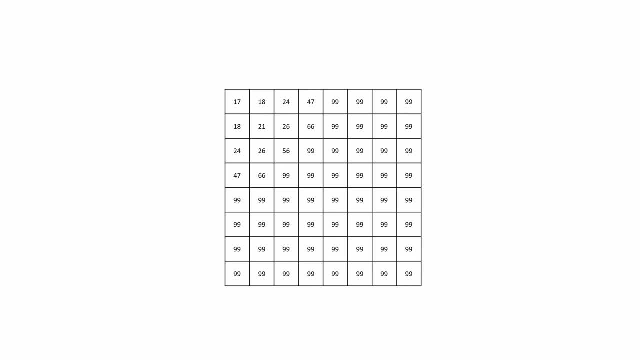 But the technique does play a part in the algorithms of other image formats such as PNG, TIFF and TGA. Without going into detail here, part of the JPEG compression algorithm involves dividing an image into 8x8 blocks of pixels. These blocks are then mathematically converted into tables of brightness and colour information. 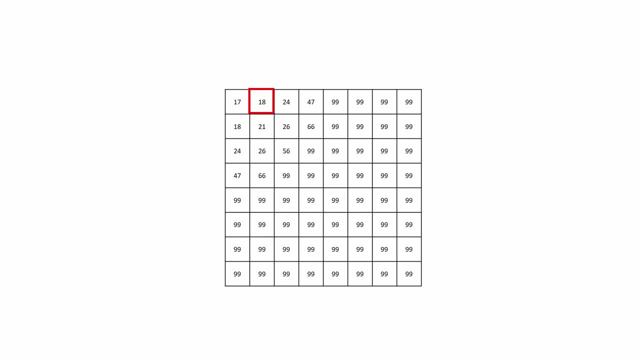 like the one shown here. These tables are then compressed with run-length encoding. It's in the nature of these tables that longer runs can be achieved by scanning diagonally and in a zig-zag fashion. To summarise, run-length encoding is a lossless compression algorithm. 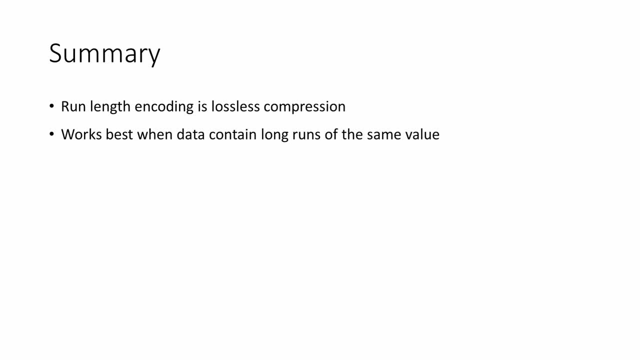 It works best on data that have long runs of the same value. For example, a black and white image of a page in a book will encode well. due to the large amount of white Run-length, encoding was used in old style fax machines. for this reason, 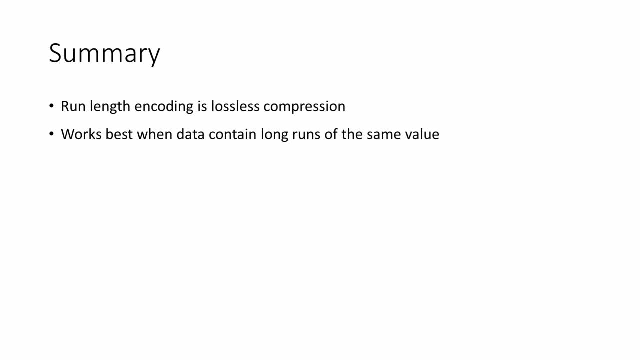 Line art images and architectural drawings that contain only a few colours, with large white or black areas, are also suitable. It's good for compressing certain other types of data as they're being collected by data logging applications. for example, Some medical scanners that generate huge amounts of three-dimensional imaging data also take. 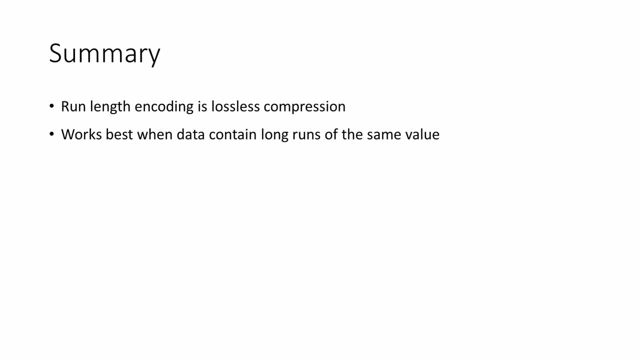 advantage of the simplicity of run-length encoding. Run-length encoding is easy to implement. Even so, there are lots of ways this might be done. For example, in some implementations the output is a one-dimensional stream of count and value pairs- The example you've just seen scanned for sequences of common pixels.